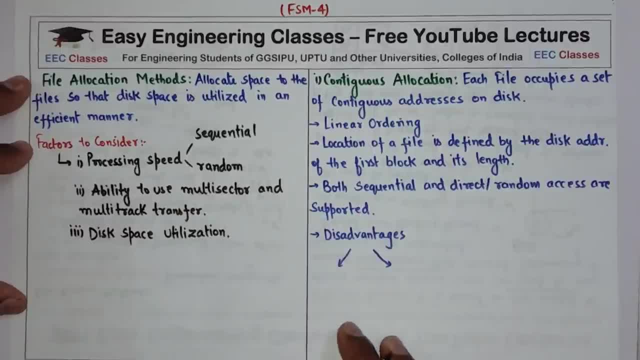 number of files can be stored in a disk. So, for example, if I have a disk size in a disk size of, suppose, 500k and one block of, say, 400k, and I have a file of 390k and I have to allocate that file to the disk. Now there are two blocks: either I can choose 500k or I can choose 400k. 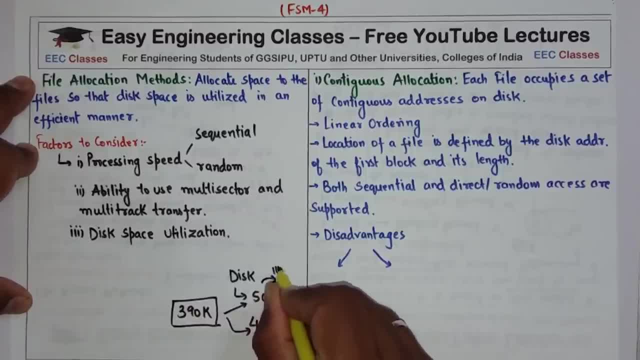 Now, if I choose 500k, that means I am wasting 110ks of memory, And if I am using choosing 400k, then I am wasting only 10ks of memory. So disk space utilization says: choose the block in which the disk space is better utilized or efficiently utilized. So this is your third. 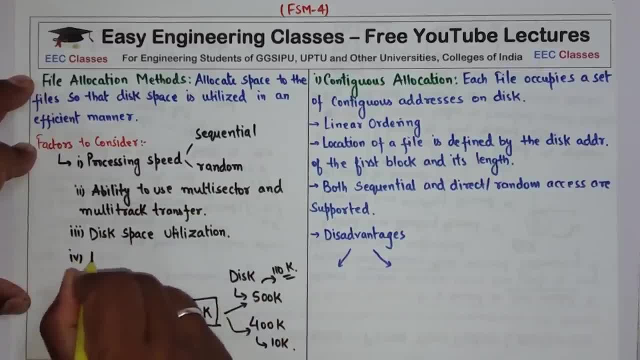 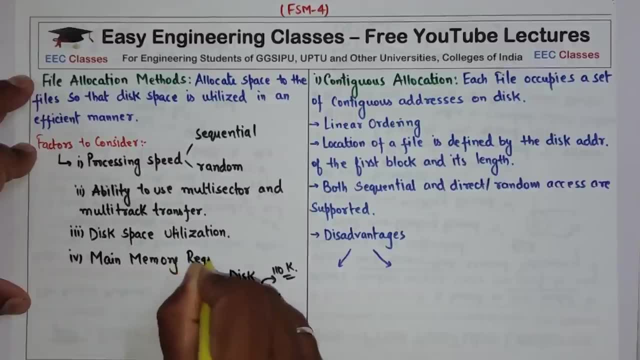 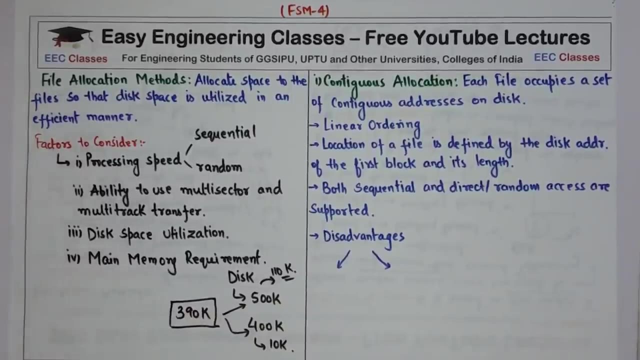 factor. And the fourth factor is main memory requirement. Now, main memory is always a constraint in any operating system, So file allocation should be such that main memory requirement is less or less. So these are some of the factors that you need to consider that an operating system should consider before. 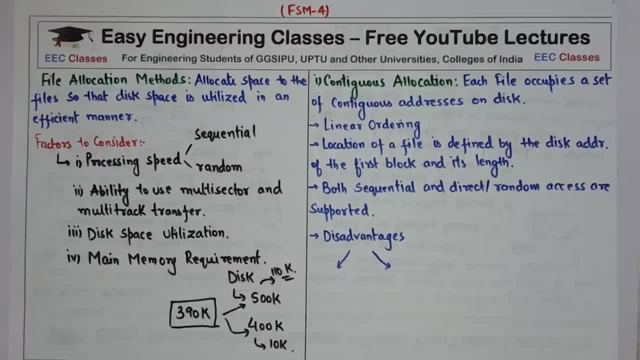 allocating a space to the file. Now, there are different kinds of allocation methods, and we will see each of those methods one by one in this video. Let's start with the contiguous allocation. In contiguous allocation, each file occupies a set of contiguous addresses on disk. 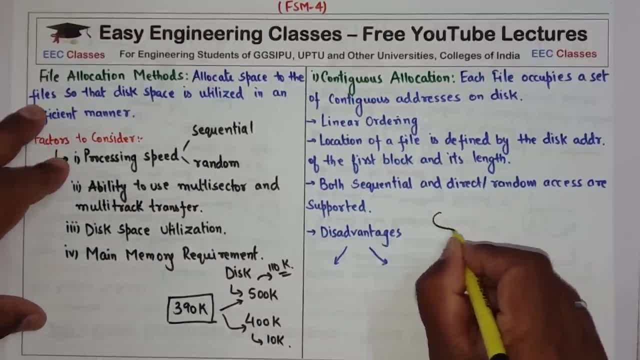 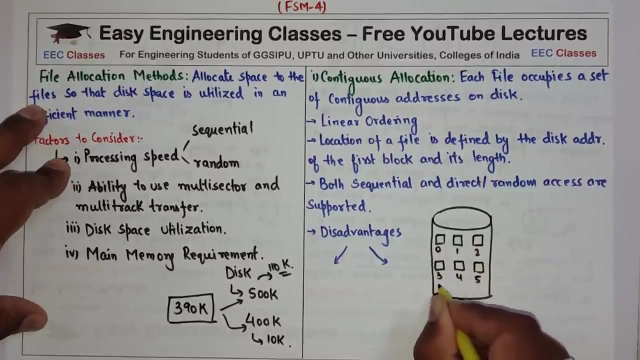 So suppose if the disk is like this: we have a disk and we have certain blocks: 0,, 1,, 2, 3,, 4,, 5,, 6,, 7 and 8.. Suppose we have a disk like this with 9 blocks numbering from 0 to 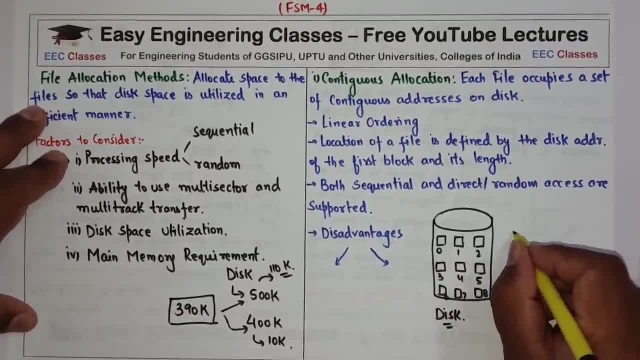 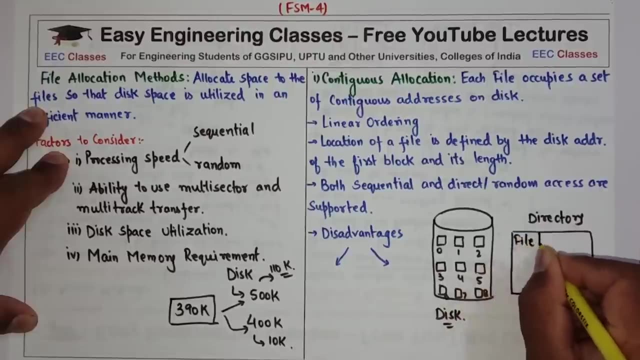 8. And we have a file directory which is used to map that which file is stored at which location. There is a directory with the file name And the starting block of the file and the length of the file. Suppose we have A start. 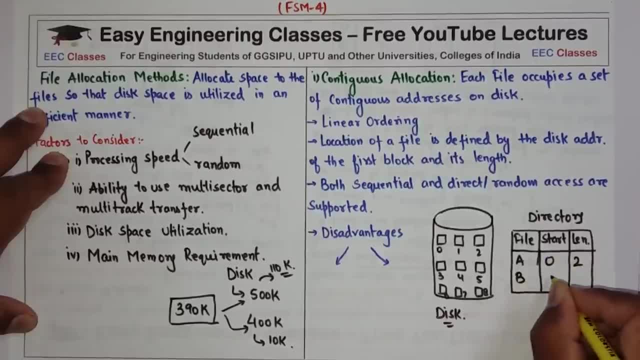 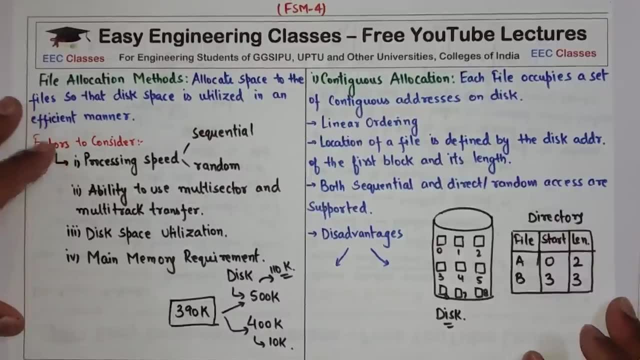 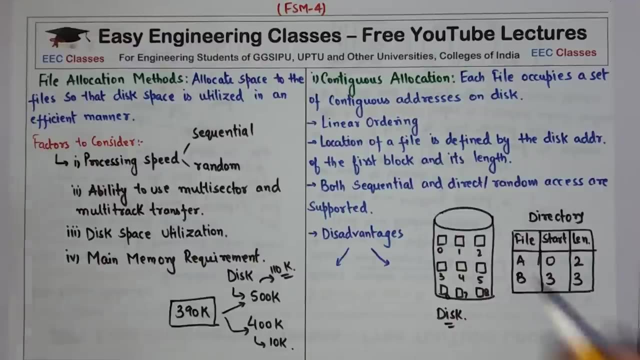 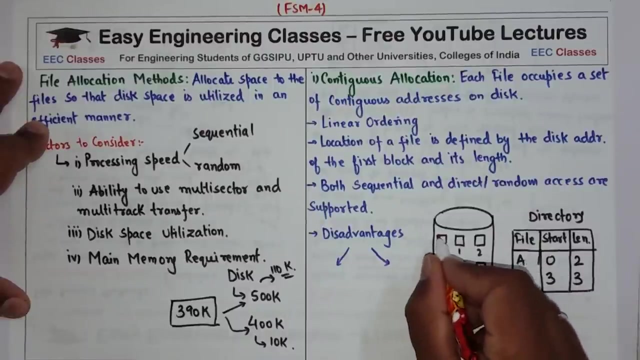 is 0 and length is 2.. And also we have B: start is 3 and length is also 3.. So it says each file occupies a set of contiguous addresses on disk. It means that if file A needs to be stored in this disk with starting as 0, so file A 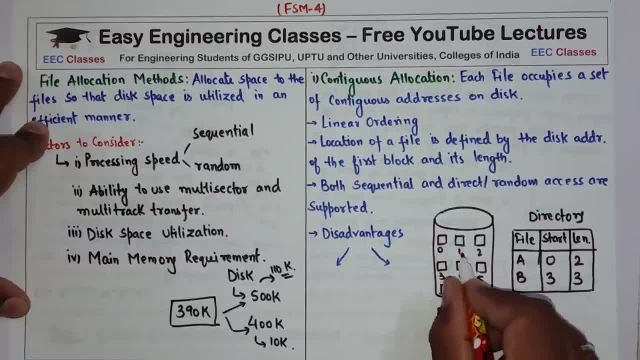 will occupy this 0 and goes up to 2 length of contiguous blocks. So the location of file A is like this: This is your file A, with starting at 0 and going up to length, which is 2.. So the first block and second block, Similarly B, starting from 3 and goes up to 3 lengths. 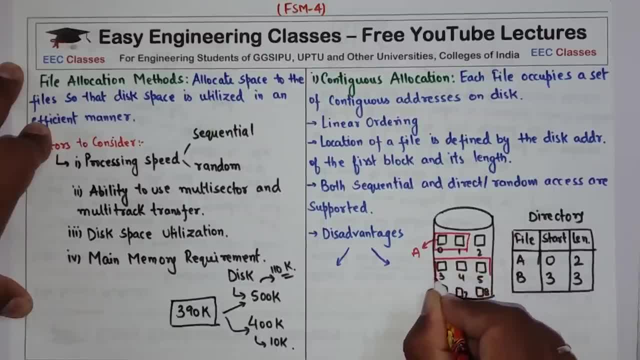 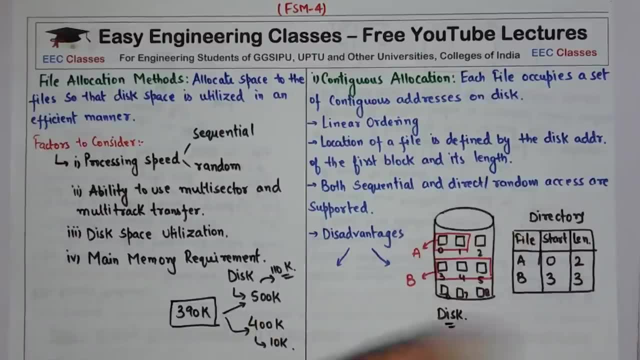 So B will be stored in a contiguous location like this. So this is how contiguous allocation works. In this, the linear ordering is used. as you can see, The location of a file is determined by the disk address of the first block, like this: 0 and its length. 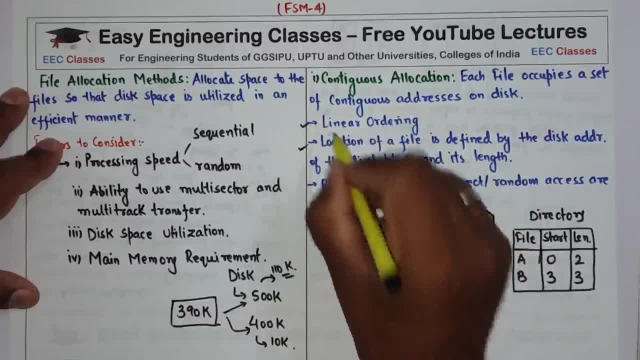 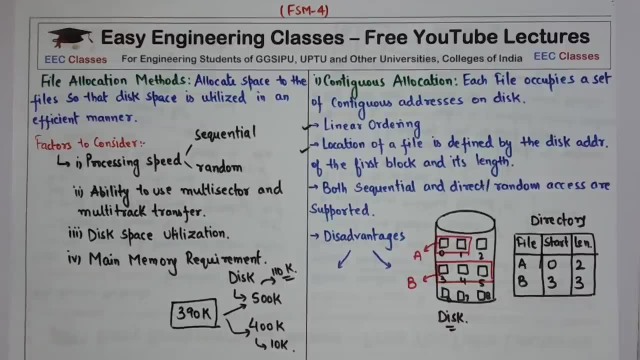 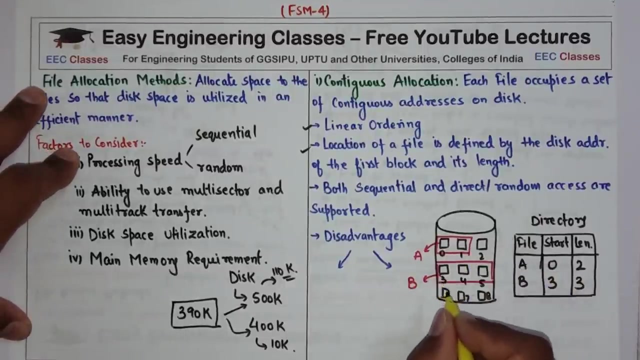 As we have already seen, Both sequential and direct random access are supported. Now let's see how sequential and random access are supported. For sequential access, file system remembers the disk address of the last block and, when required, reads the next block. So for sequential access, the file system just remembers the last block that it has. 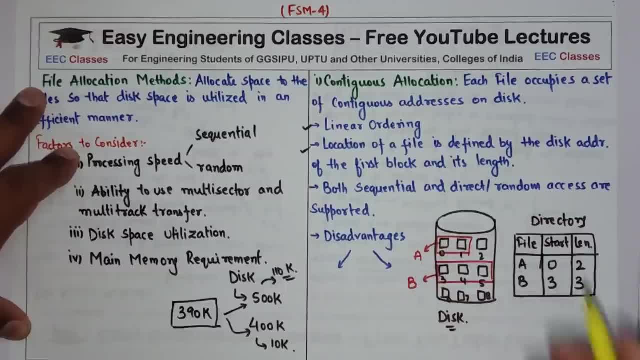 read and then reads the next block. So an example of sequential access is the file system Будет and starts from reading the next block, but for random access. for random access, let's say the file starts at block b and it needs to access ith. 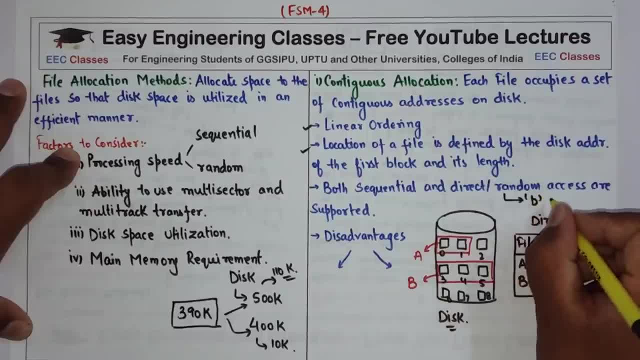 record in that block or in that file. so for random access the address or location will be b plus i. for example, let's say a user wants to access second record of file b, so what? it will be three plus second record, that is zero. one first record, second record, that is. 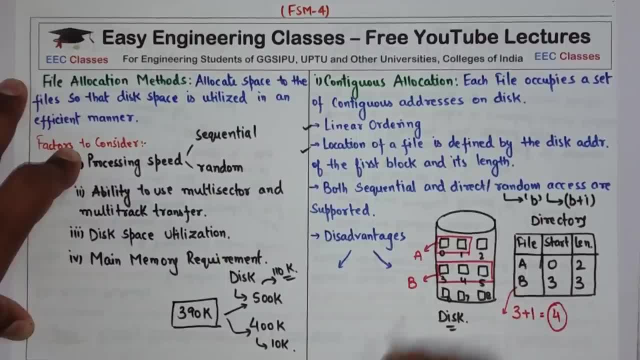 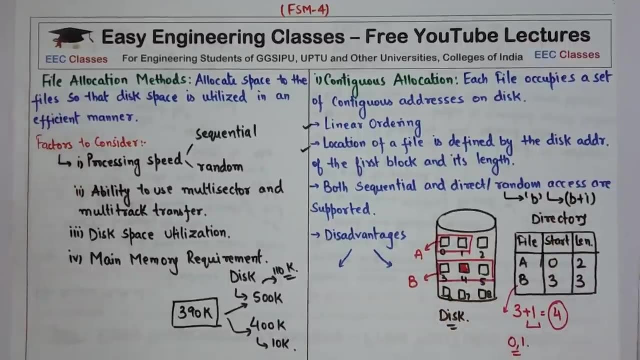 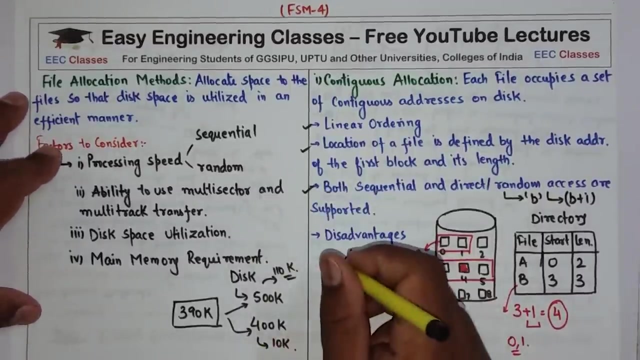 four, so it will directly access this particular record. second record: i have used one because i want to use all orders. am using the index from zero, So that is how random access is also supported in the contiguous allocation. But there are certain disadvantages of contiguous allocation. 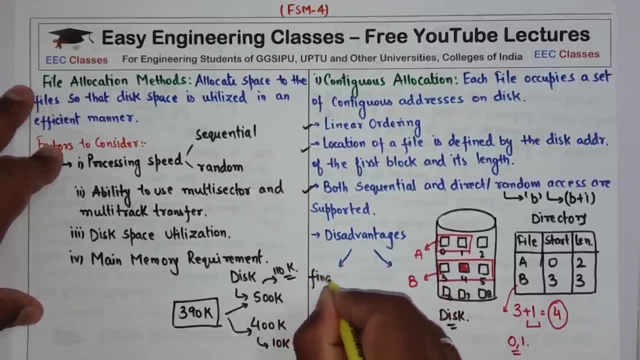 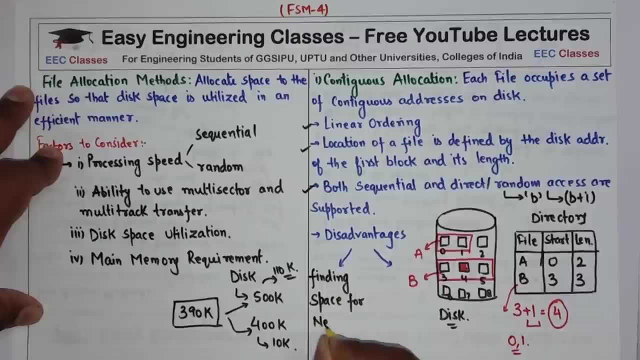 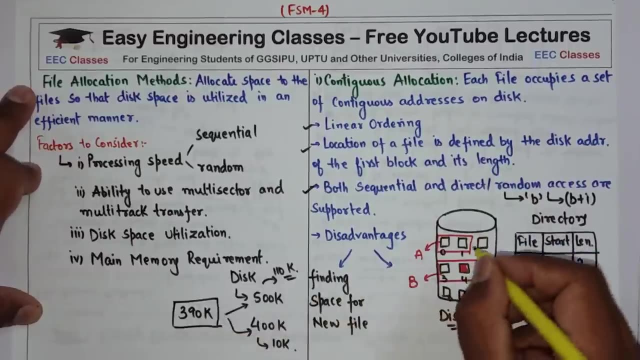 The first disadvantage is finding space for new file. Finding space for new file is very difficult in contiguous allocation methods because you have to keep track of the free blocks. Let's say, after allocating A and B, this second block is free. So we need to keep track how many blocks, where it is stored and when it is free. Then the second disadvantage is external fragmentation. This is the biggest disadvantage of contiguous allocation. External fragmentation: This is the biggest disadvantage of contiguous allocation. One variation of contiguous memory allocation technique is dynamic storage allocation And, as we have already seen in the previous videos, there are three different types of. 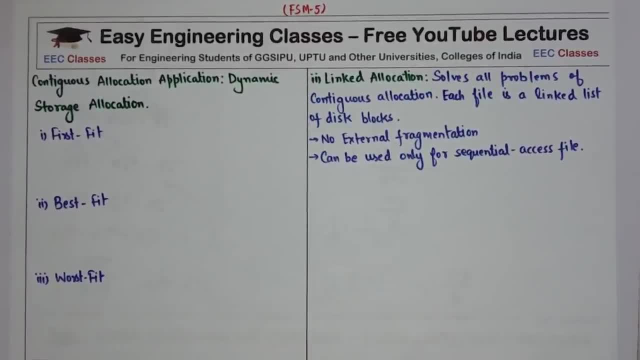 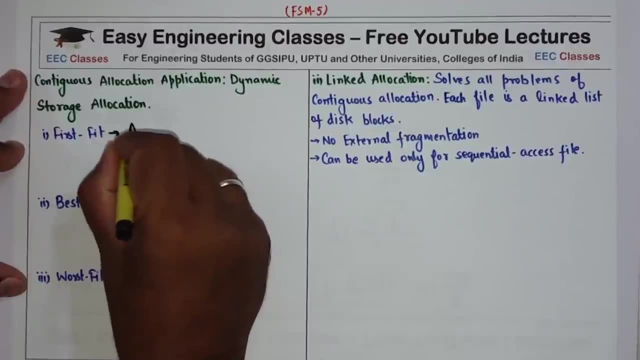 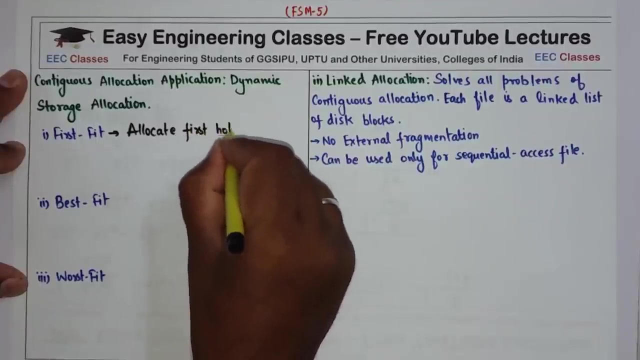 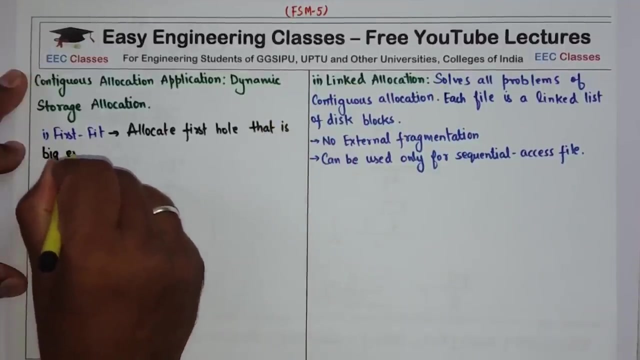 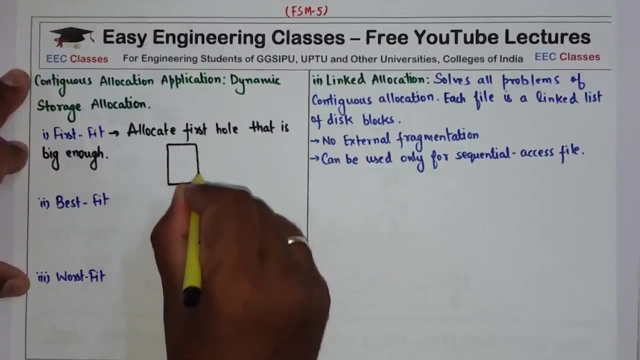 techniques. First is first fit, best fit and worst fit. So what is the meaning of first fit is allocate the hole, that is, allocate the first hole, that is big enough. Now, for example, let's say I have two different holes, one of size 400K and another is of 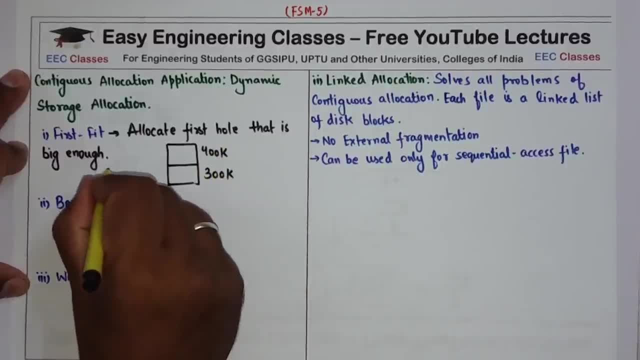 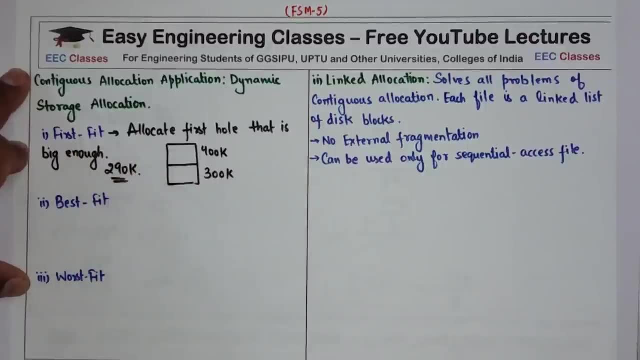 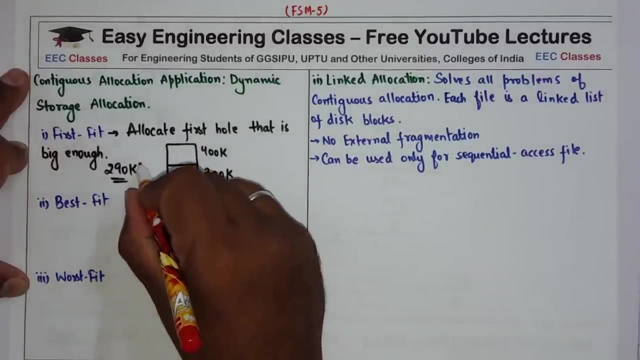 size 300K And I have a file of 290K to allocate, Then I have a file of 290K to allocate. Then, according to first fit, it should be allocated to the first hole that is big enough, And the first hole which is big enough for this file is 400K. 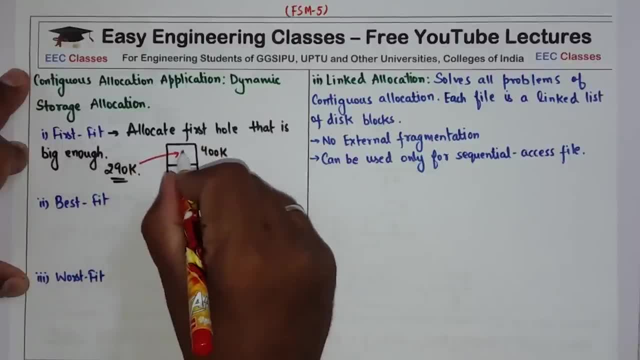 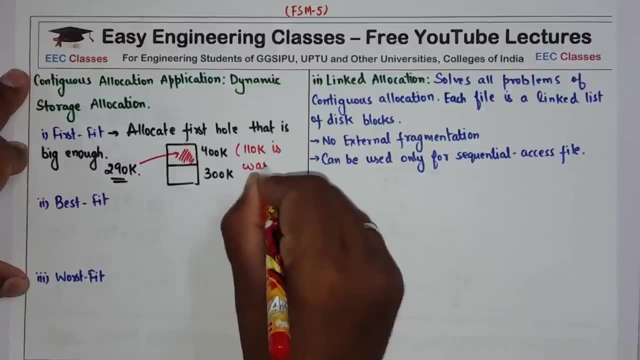 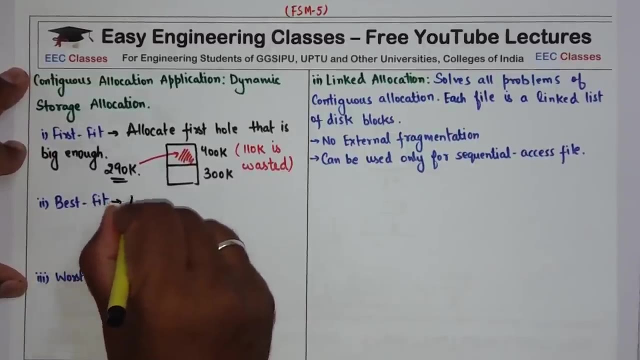 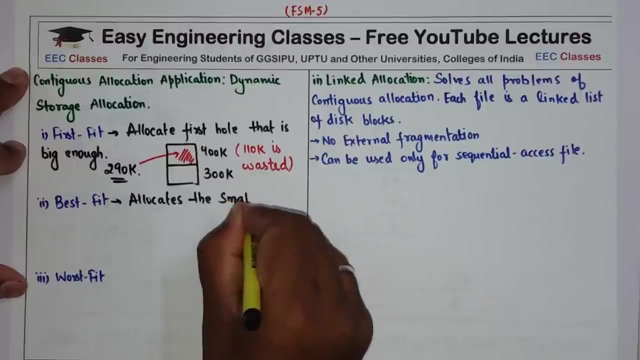 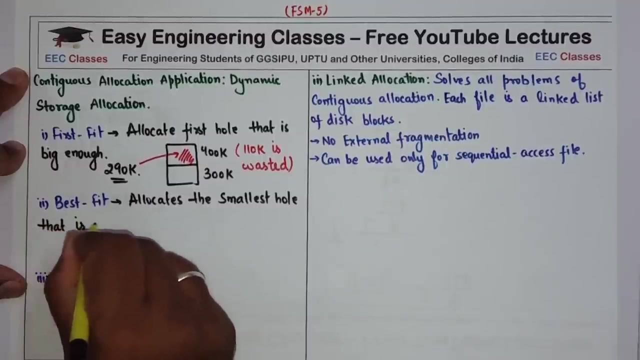 So in this, according to first fit, this 290K file will get allocated in this area And, as you can see, 110K is wasted in this. So this is your first fit. Then we have best fit. It allocates the. it allocates the smallest hole that is big enough for the file. 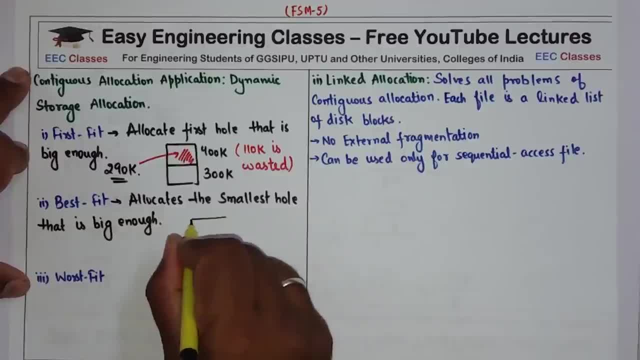 Now let's consider the same example. We have three blocks now, Let's say One block, Two blocks: One is of 300K, Another is of 400K And last is of 290K exactly, or 298, let us assume. 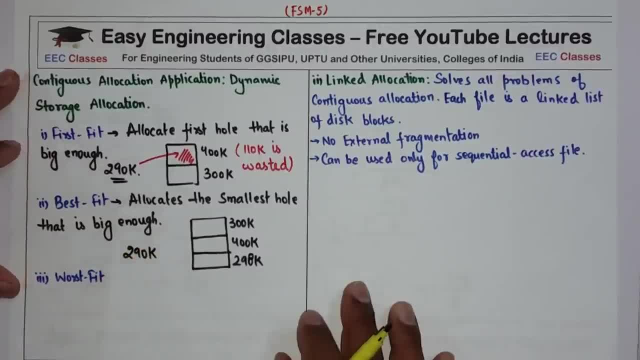 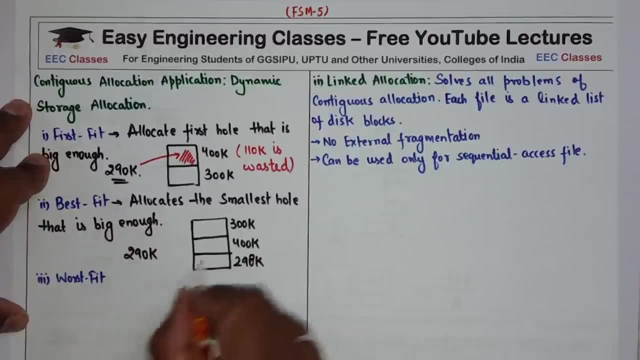 And we have a file of 290K to allocate. Now let's see, we have to find the smallest hole which is large enough to hold this particular file And, as you can see from this, 300K also hold 400K, also 298K. 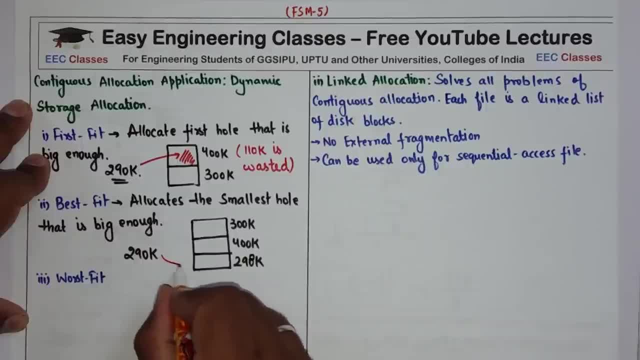 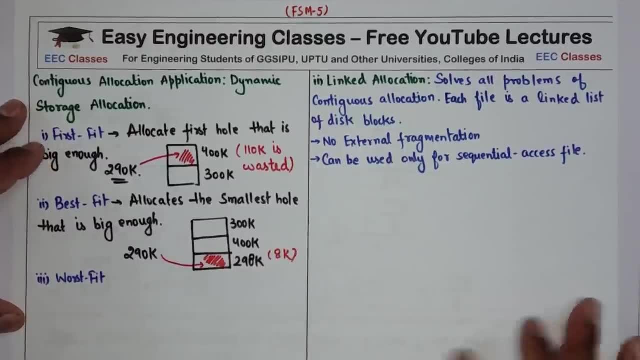 And out of this, three, which is the smallest, 298K. So this file will now gets allocated in this space And in this only 8K is wasted. So that is your best fit. Then we have the worst fit. Worst fit means allocate the largest hole. 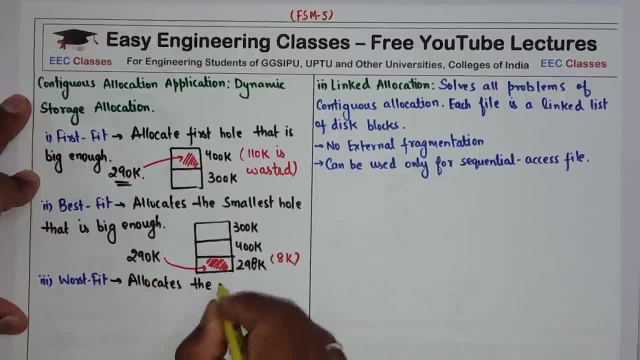 It says allocates the largest hole. Okay, Okay, Okay, Okay. Now let's consider the same example. One is of 300K, Another is of 400K, And then we have 298K, And the file is of 290K. 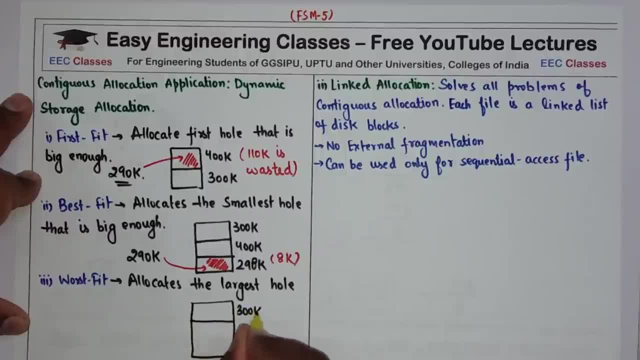 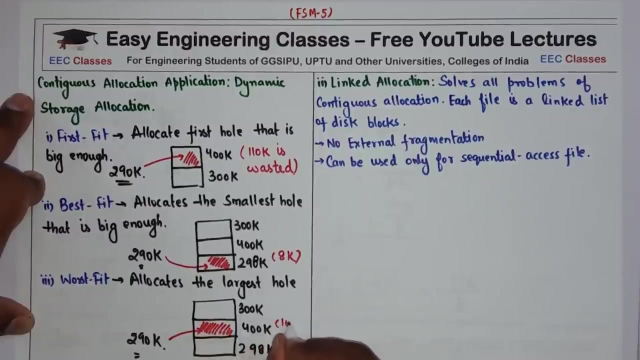 Now, as per worst fit, we have to allocate the largest hole, which is 400K, And in this, 110K of memory is wasted. Now, if we see each first fit According to first fit, this will get allocated to this. only 10K is wasted. 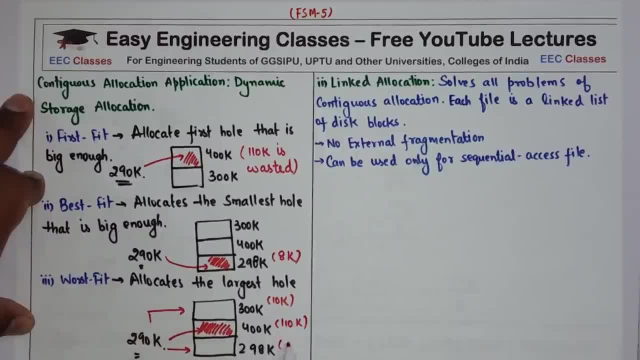 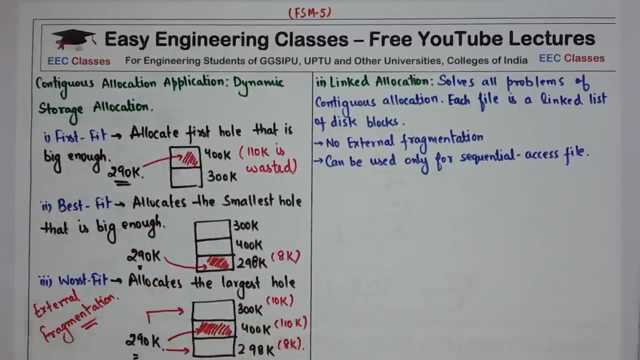 According to best fit. this will gets allocated to this. only 8K is wasted, But all of these algorithms will suffer from external fragmentation. Okay, Okay. So this is the application of this contiguous memory allocation. Next we have in this topic is linked allocation. 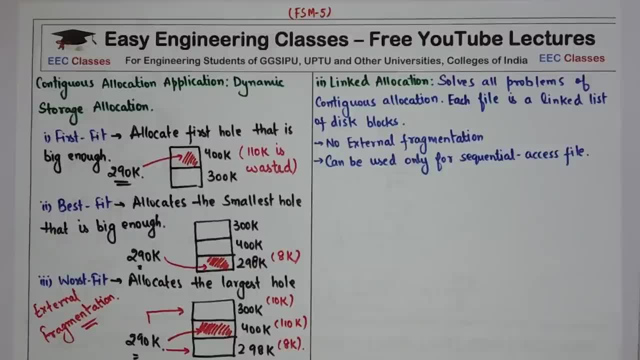 Linked allocation solves all the problems of contiguous allocation. In this, each file is a linked list of disk blocks, So it is now not necessary that we have to have a contiguous address for a file to be saved, And we can have scattered blocks and each block should be linked with the other block. 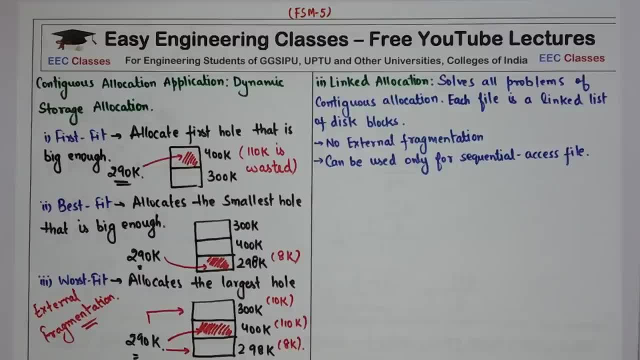 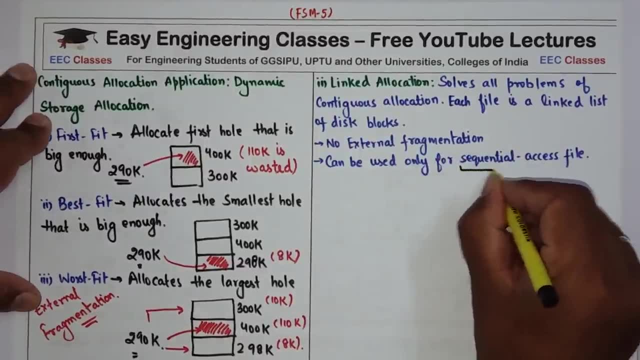 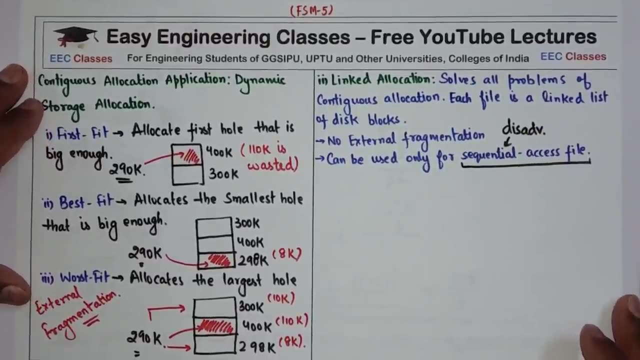 And in this there is no external fragmentation. But the disadvantage is it can be used only for sequential access of file. Now, this is the biggest disadvantage of linked allocation. Now let's see one example of how linked allocation works. Now let us assume that we have a file. 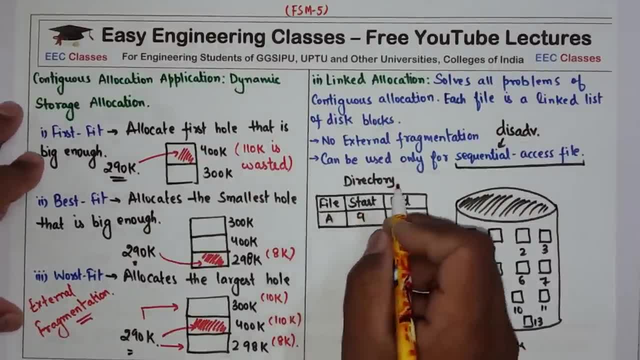 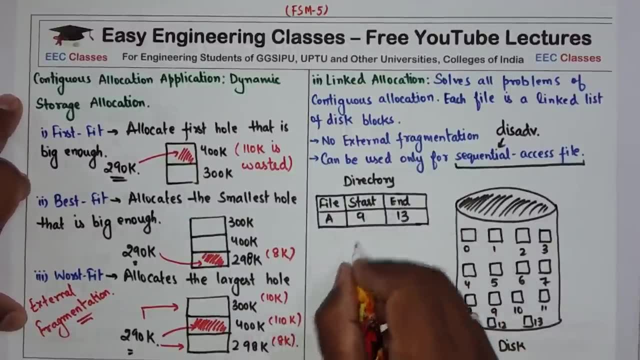 Now, let us assume that we have a file. Now, let us assume that we have a file. Now, let us assume that we have a directory like this, where we have one file, a starting location is 9 and ending is 13.. So how this will be stored in our disk with the help of linked allocation is now we know. 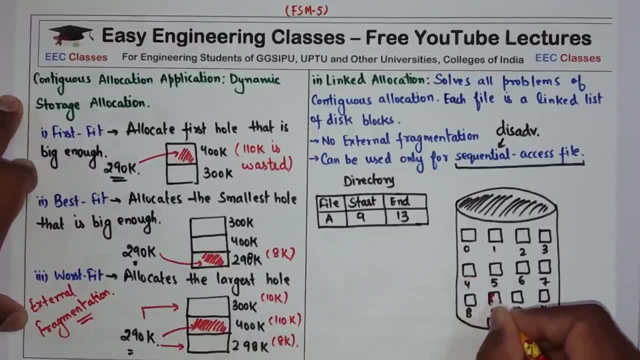 that the starting is 9.. So this pointer will be linked with this 9th block of the disk And suppose after 9.. The location or the block that is linked is 4.. So it will have a pointer like this: 4.. 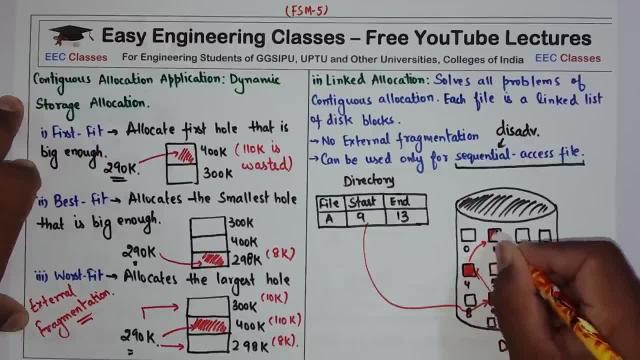 Then from 4 it can be 1.. From 1 it can be 6., 11. And the last is 13. So 11 will be linked to this 13 and also we will have a pointer from this end to this. 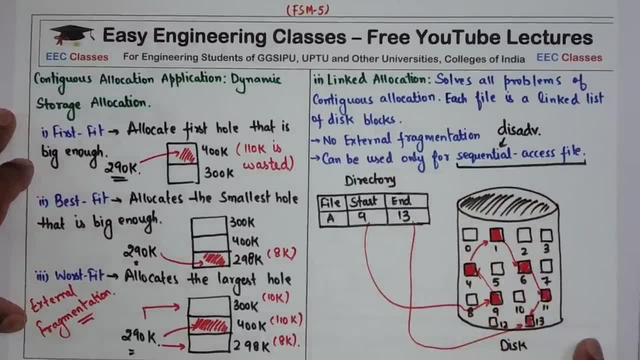 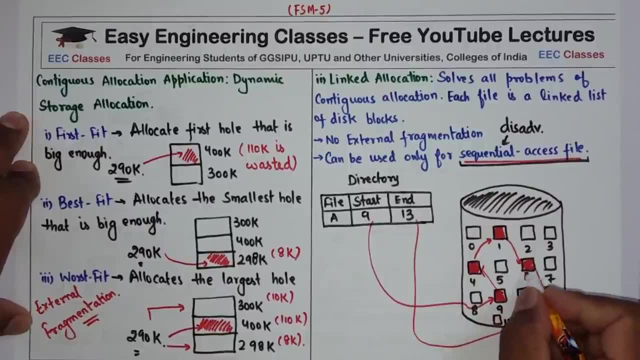 13.. So that is how this linked allocation works. But the disadvantage is there is no sequential access, Because if I have to access directly 6, then I need to go from the starting location. Then only I can access this 6.. Next type of allocation technique is indexed allocation. 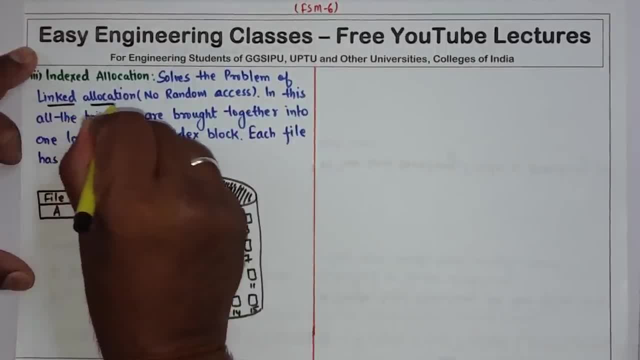 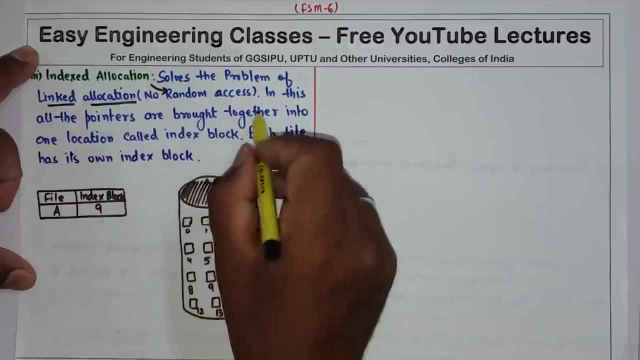 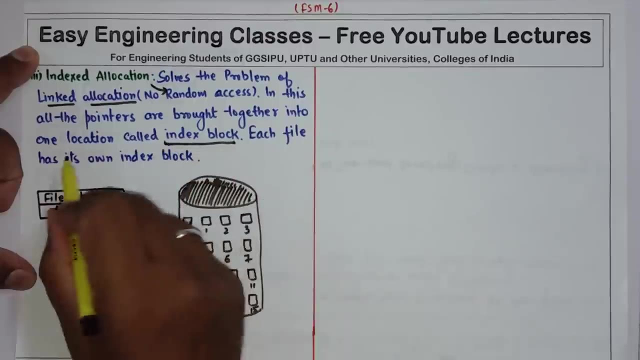 It solves the problem of linked allocation, and the problem with linked allocation is there is no random access. But index allocation allows random access. In this all the pointers are brought together into one location called the index block, and each file has its own index block. 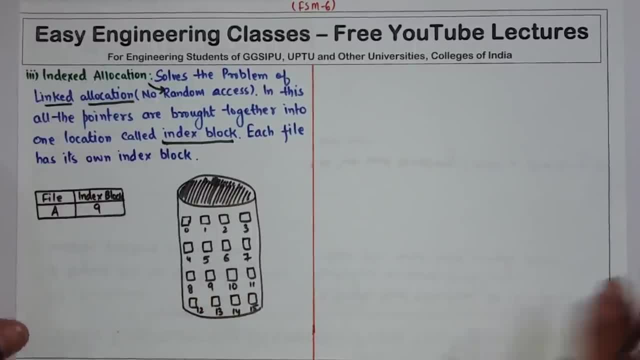 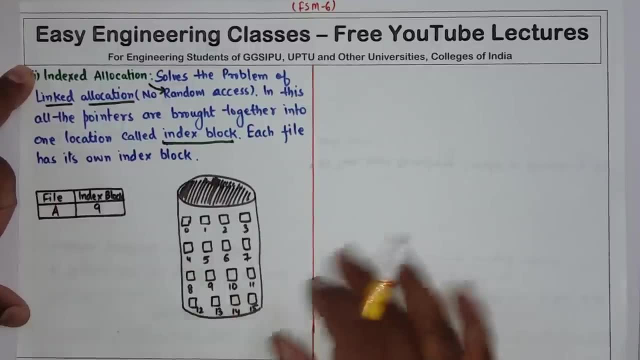 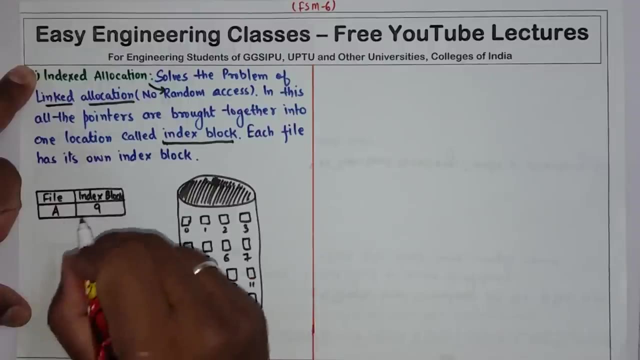 Now let me explain this to you with the help of an example. Let suppose there is a directory structure here like this with file a and the index block is 9. So this is your index block And all the pointers of this file are present in this index block. 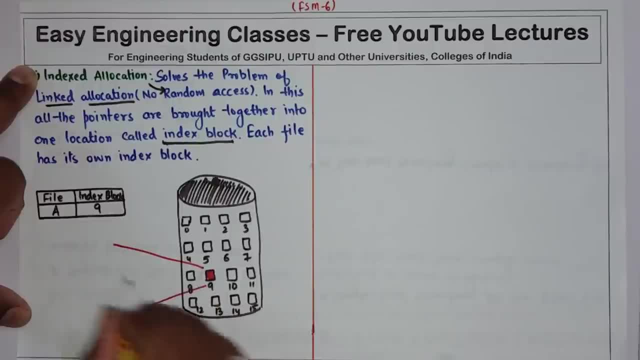 So this index block will look like this. It will have all the pointers say 4,, 2,, 3,, 7, it means that file a is stored at location 4,2,, 3 and 5.. 7 and the information of this storage area is present in this index block. so 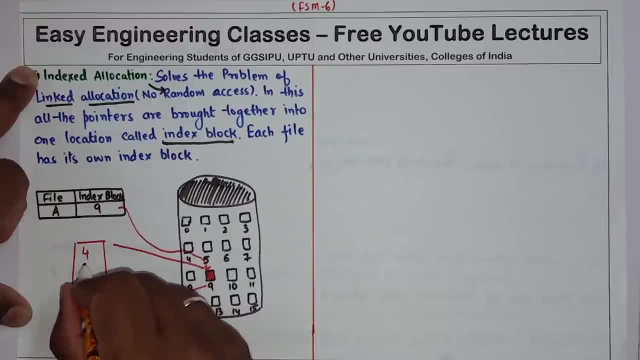 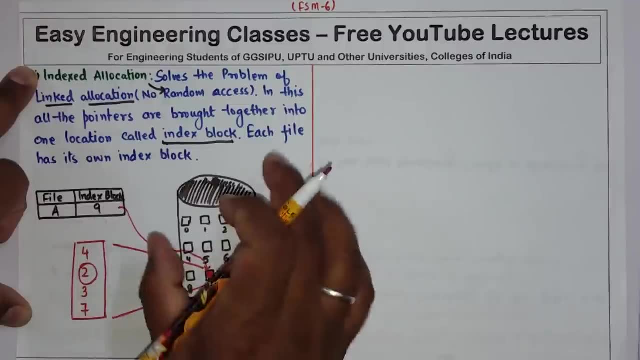 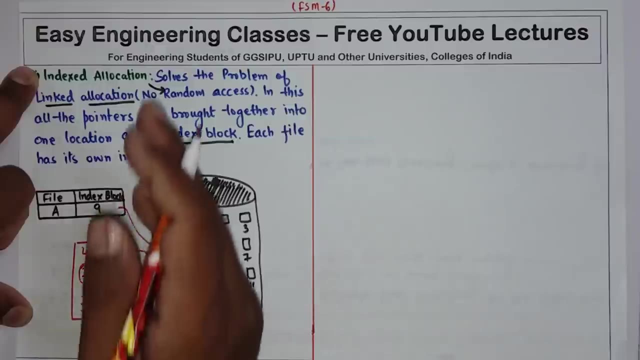 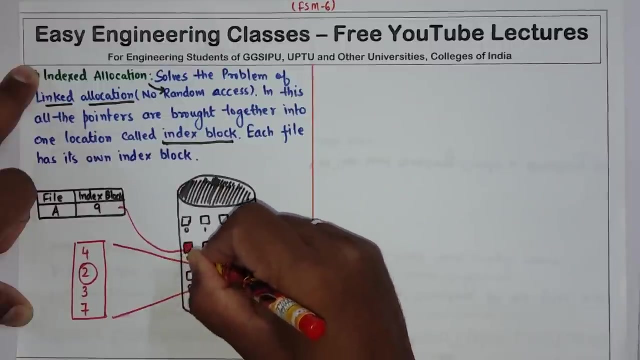 now, after this, what happens if I have to access this block 2, then what I need to do I need to find the index block, go there and from this I can directly access the second block. so that is how it solves the issues of linked allocation. now, from 9, I have a link to 4, so you can join and show this from 9. I. 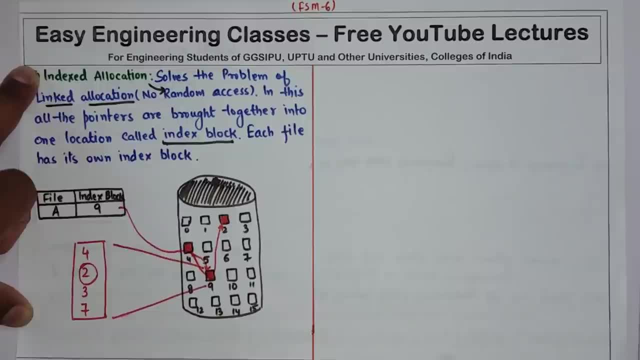 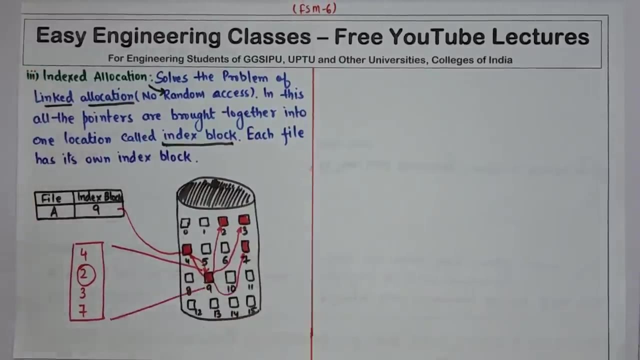 have a link to. then from 9 I have a link 3 and 7. so at these locations file a is stored. so this is about the indexed allocation. thank you for watching this video. please subscribe to my youtube channel for more such tutorials. thank you.